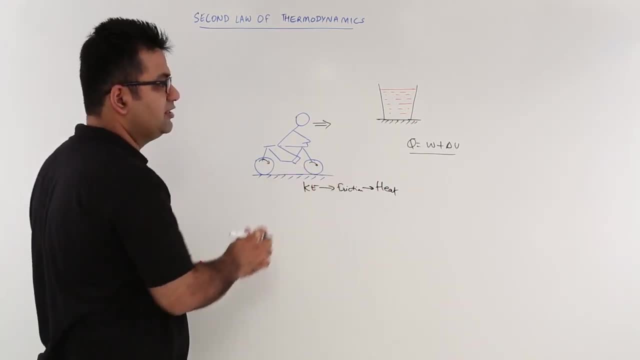 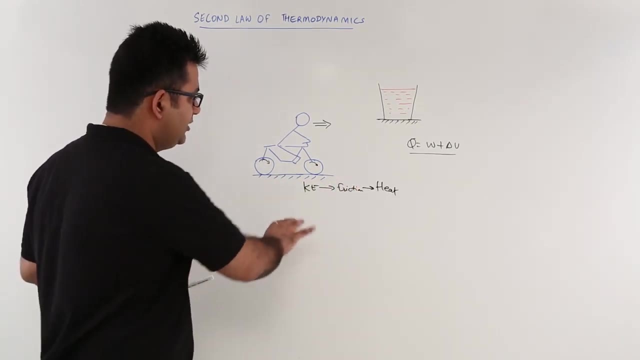 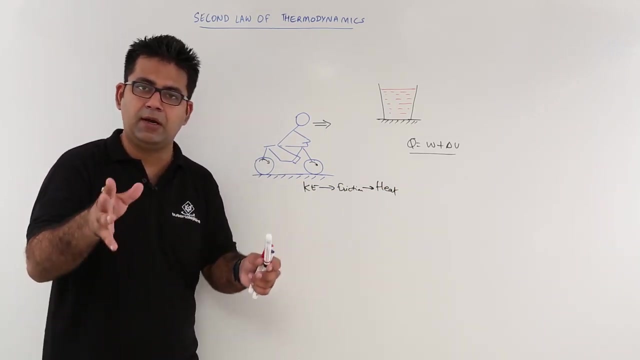 into the surroundings. Okay, Now, this is a process which is happening in this particular order Right Now. as per the first law, this process would stop when the atmosphere, that is, the system in the surroundings, will come under an energy balance. 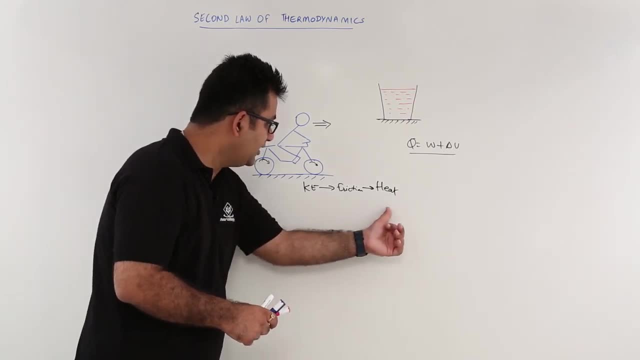 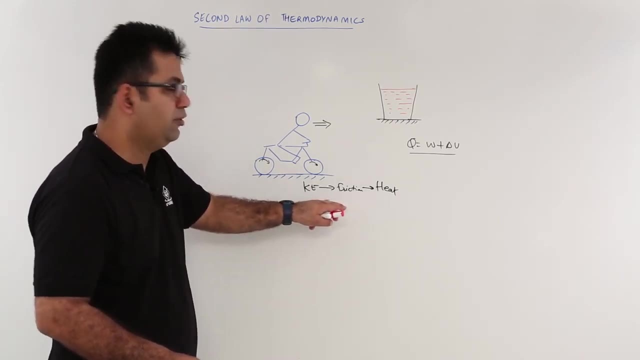 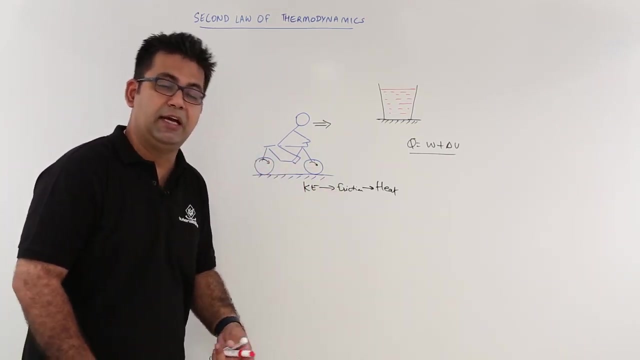 Okay, Now if I proceed in the, you can say the reverse order. If I say I develop heat, then that heat converts into friction. That friction will convert into the kinetic energy or the motion of this bike. again, Is that possible? That's not possible. 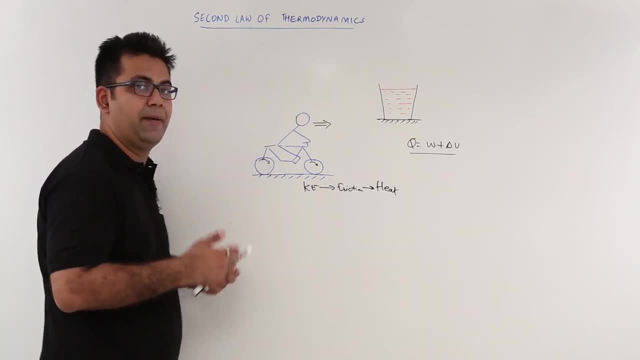 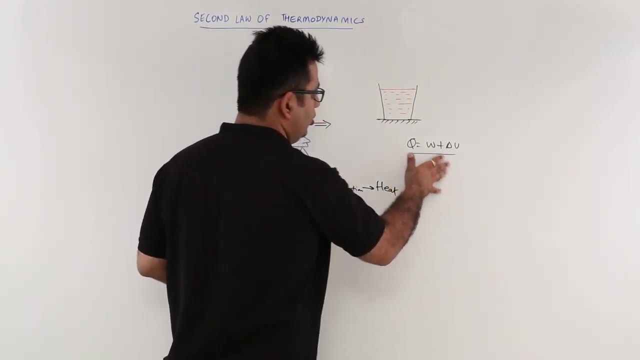 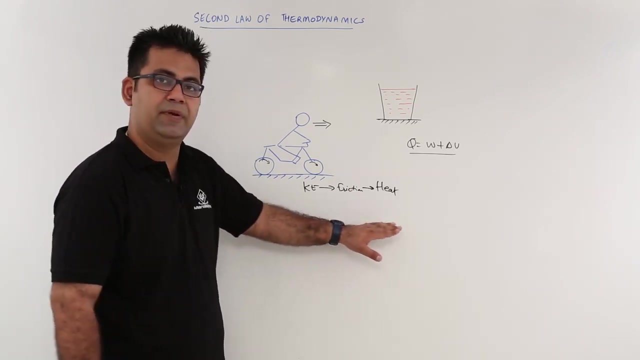 Because you cannot have the reverse order of this process happening on its own. So this brings us to a question that the first law is only giving us that this process is occurred, or this process has occurred, And after the occurrence has been complete, you get a certain balance. 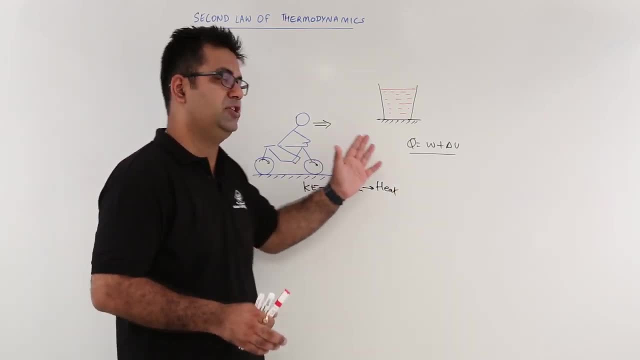 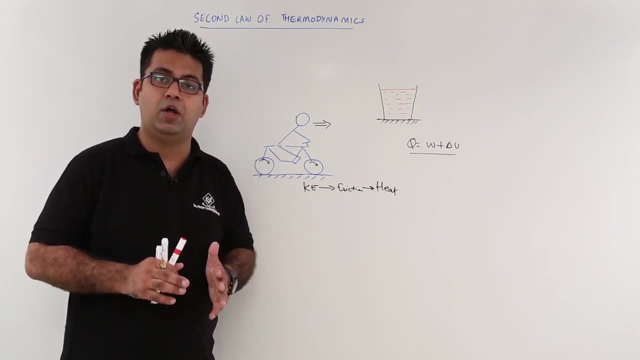 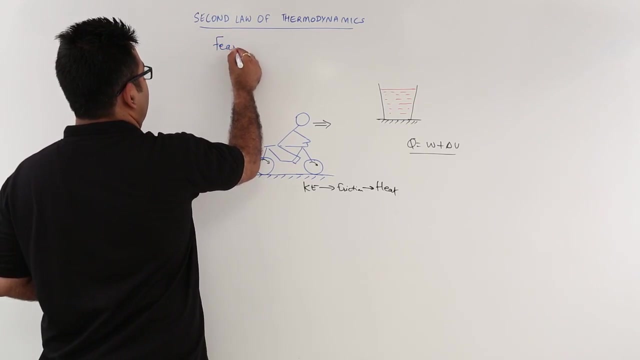 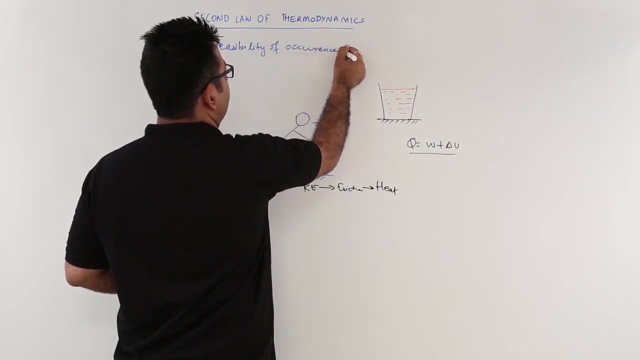 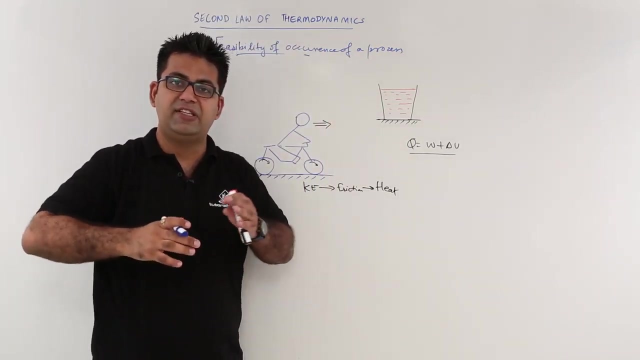 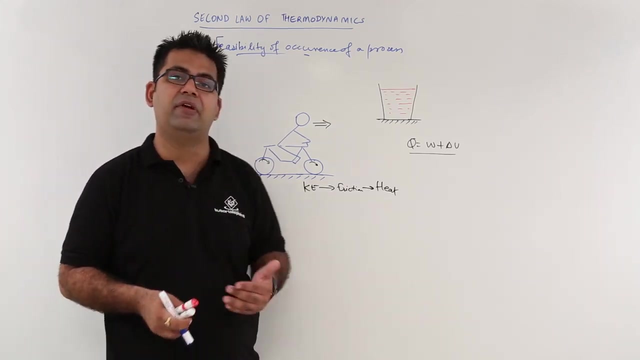 in the whole system and surrounding environment for energy: Okay, It does not tell us whether this process will occur or not occur. Okay, That is called the feasibility of the occurrence of a process. Feasibility, Okay, And the feasibility. by feasibility we mean that whether this process will occur or not, And by experiments we have come to know. 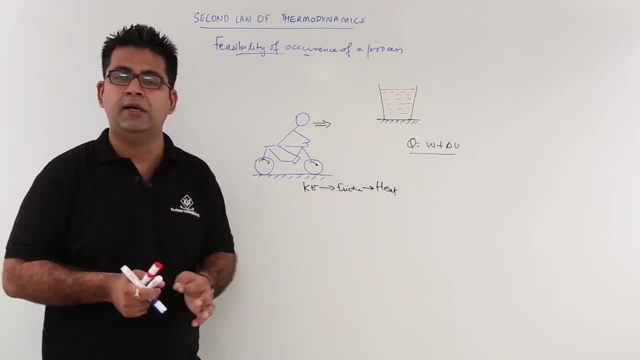 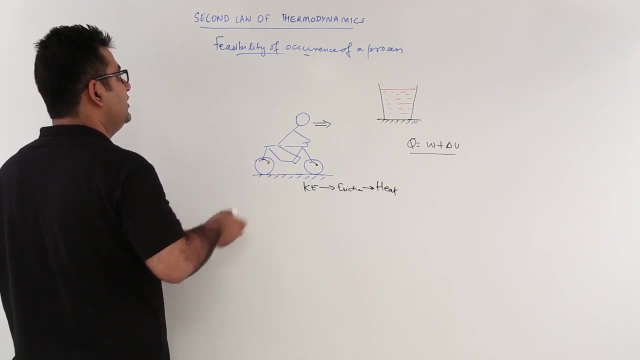 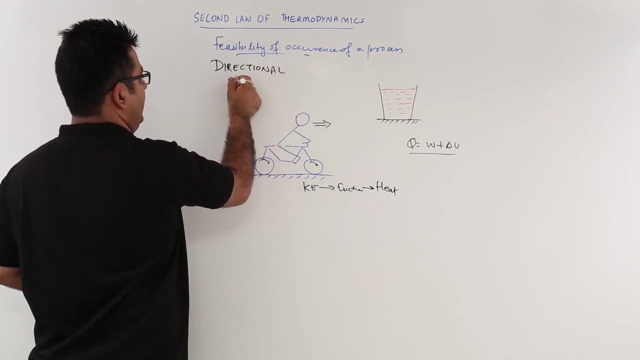 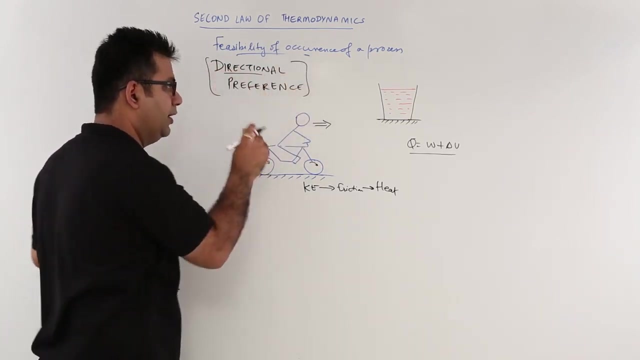 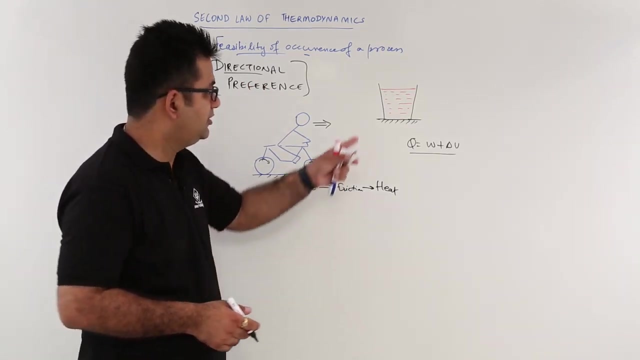 that the processes have a certain directional preference for their occurrence. So this is a pretty important word: that the processes have a directional preference. A directional preference means they only prefer to proceed in a particular direction only. They cannot proceed on its own in the reverse direction. Okay, So if you take the example of this figure also, this is a glass. 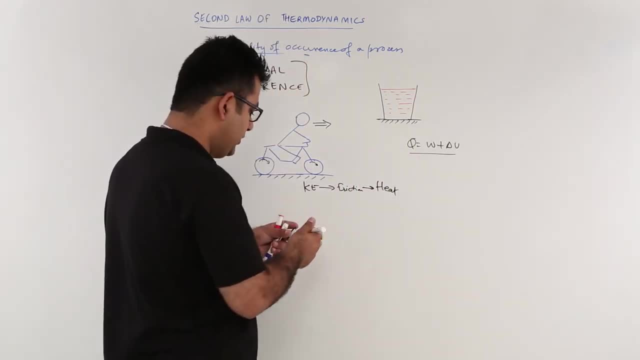 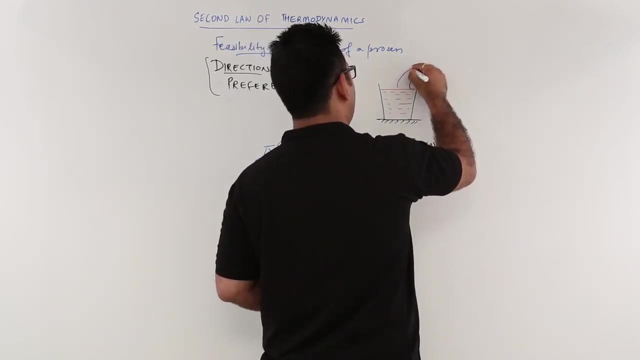 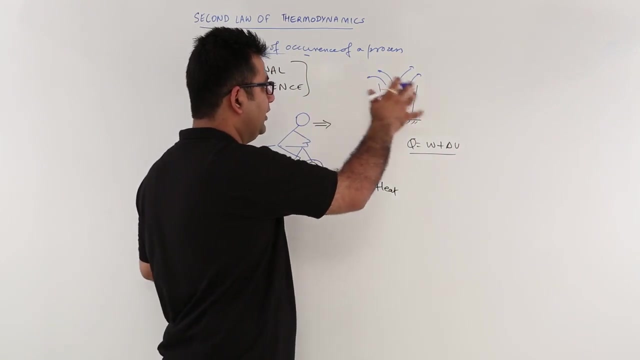 which contains some hot liquid. Now what happens is, as per the first law, you will have some- you know- heat which will go out into the atmosphere like this, okay, and this heat out flow will stop till there is an equilibrium which is set up, you know, around this liquid on the 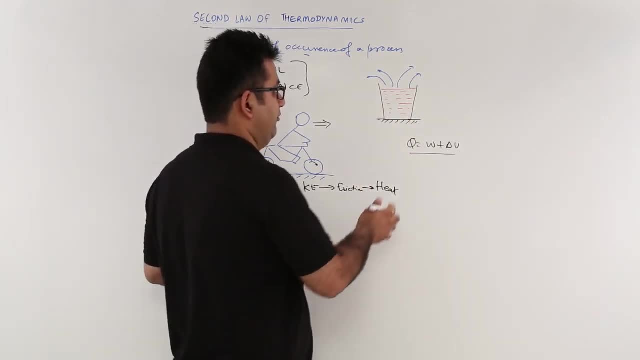 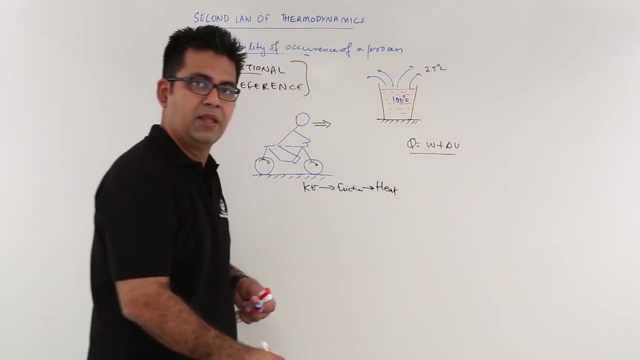 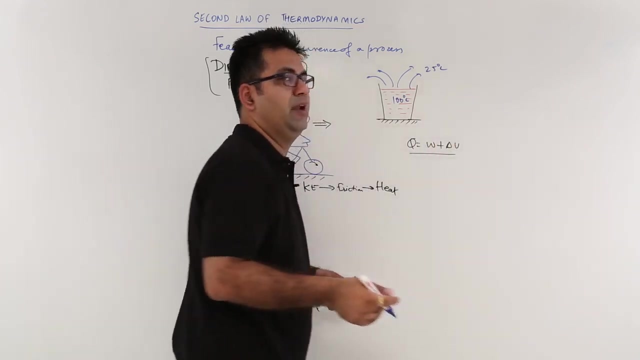 surroundings, okay. but if, let us say, this hot liquid is at 100 degree Celsius and surroundings are at 25, so the immediate vicinity of this liquid, you know, will, till the time you have an equilibrium temperature, your heat flow, your energy flow will stop okay. so you need. 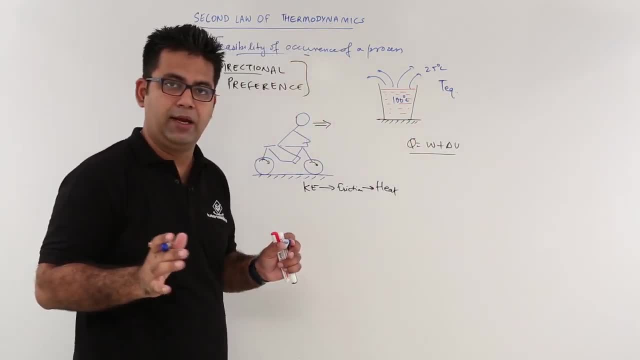 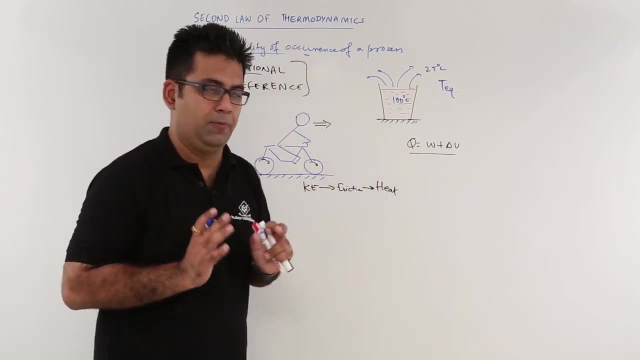 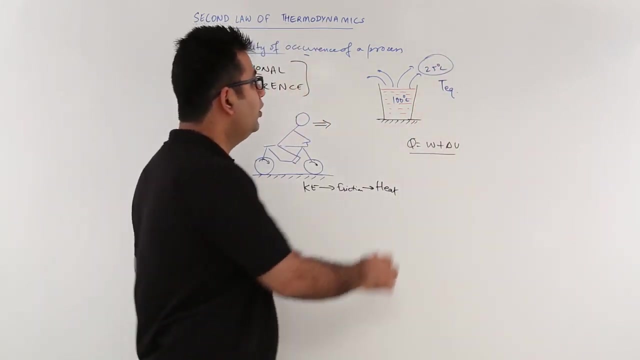 to achieve an equilibrium temperature right in order to bring the equilibrium conditions for this to stop the energy interaction. now, if you proceed in the reverse order, that is, if you extract heat- heat from the surroundings, can you attain 100 degree Celsius of hotness of this liquid? 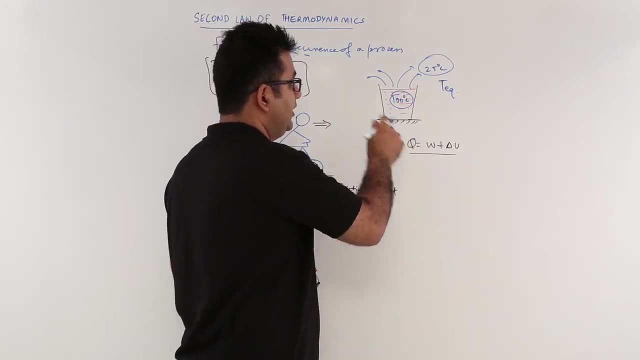 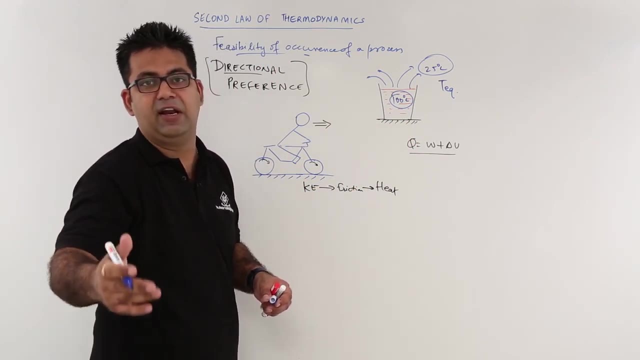 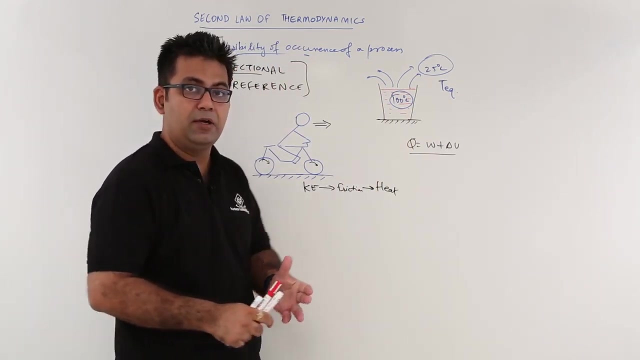 again: no, you cannot. this means that this process of heat rejection from a hot liquid can only proceed in a preferred direction, that is, from this hot liquid to the- you can say- outer, colder surroundings. but if I am able to extract, or if I extract heat from the surroundings and 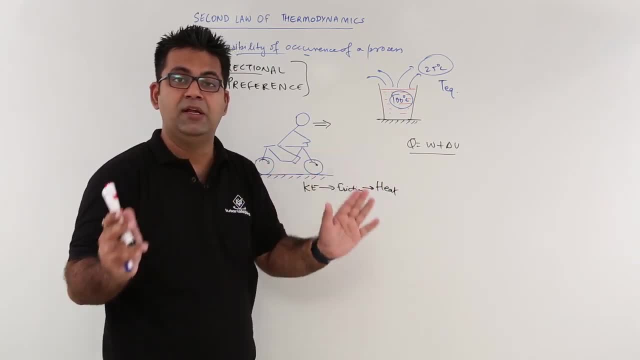 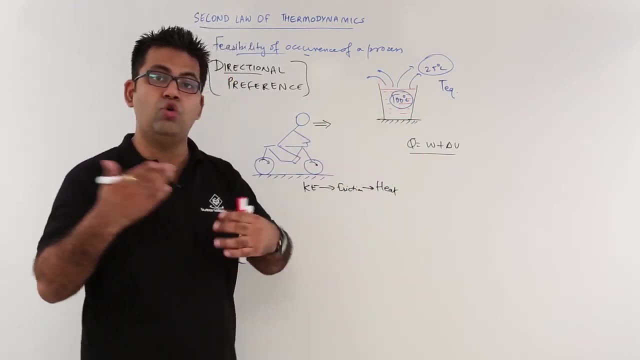 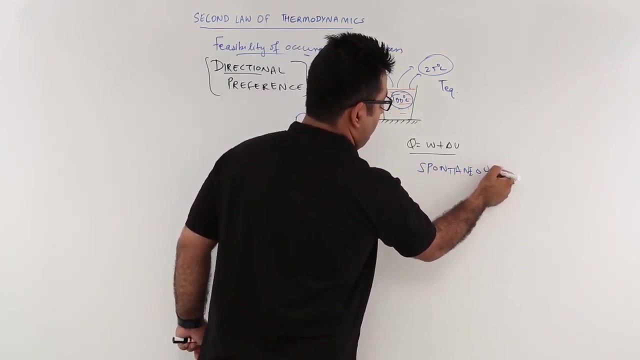 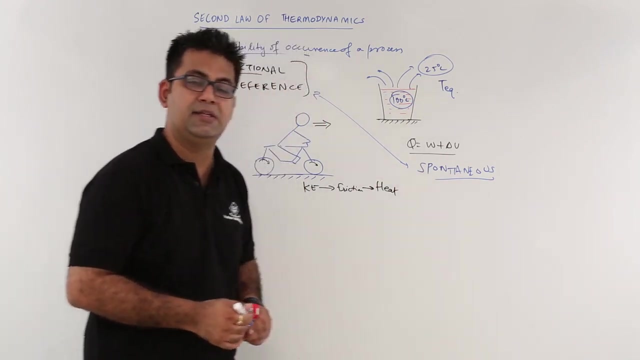 I put it back into the liquid on its own and nobody, no external forces applied. this is outflow of heat is happening on its own, and that on its own we mean that the process has to be spontaneous. okay, so now we are going to combine these things. so: spontaneous occurrence of any process. 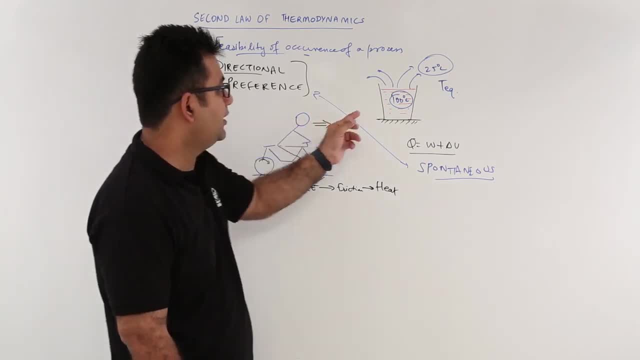 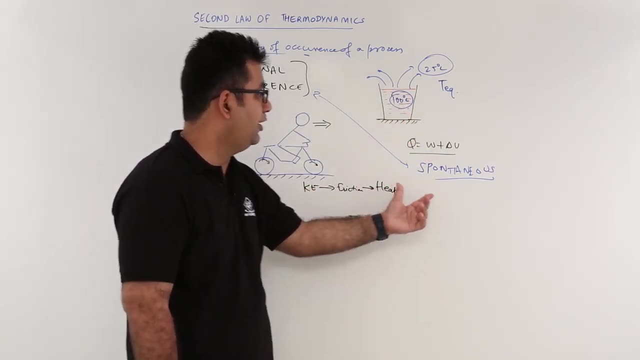 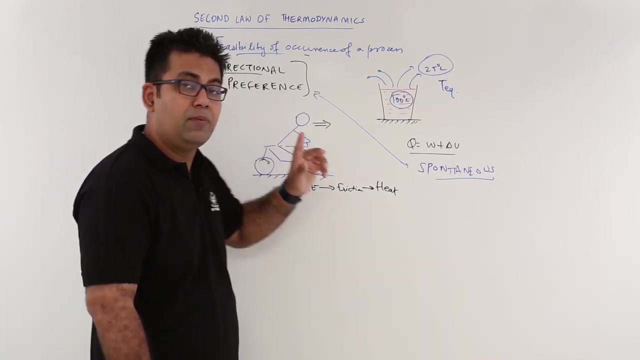 will have a directional preference. If this occurrence of heat flowing out from 100 degree Celsius liquid into 25 degree Celsius of air, this is a spontaneous process which occurs on its own and it occurs only in a preferred direction. But if I talk about the reverse, 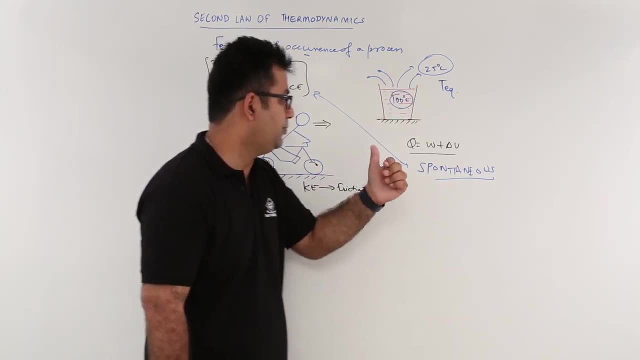 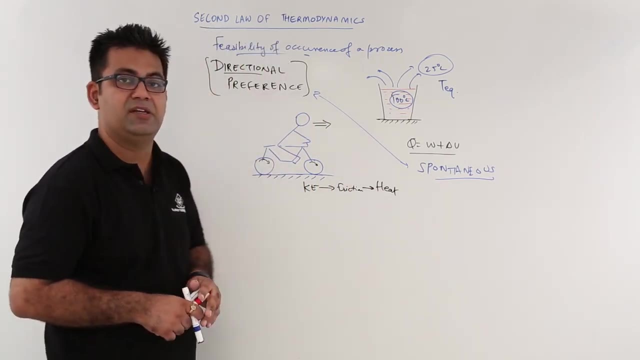 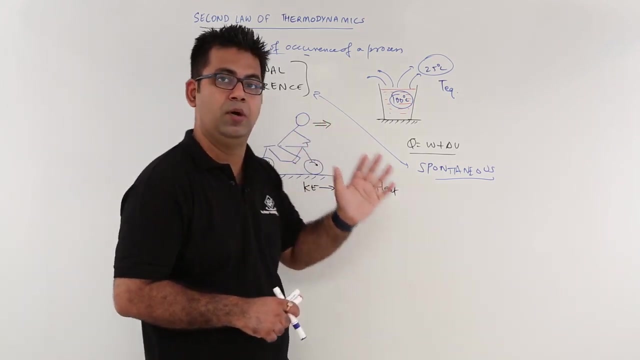 of it, that is, heat flowing from 25 to 100,. it is not spontaneous means it will not happen on its own, And this means this directional preference is a very, very important concept to understand And this is not taken care of by the first law. So this is a limitation. 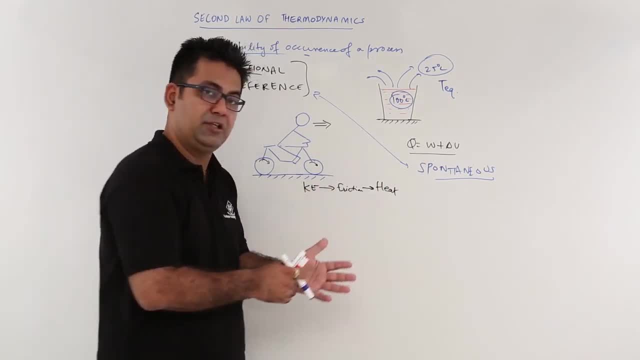 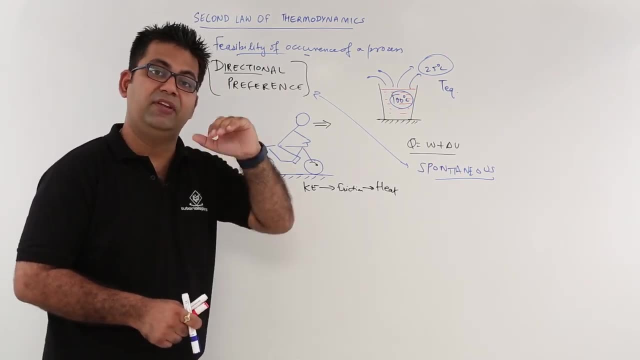 of the first law and to eliminate that limitation of the first law, we come to the study of second law of thermodynamics, which talks about this feasibility that, whether this process would occur or not occur. So this is what we cover in this video.